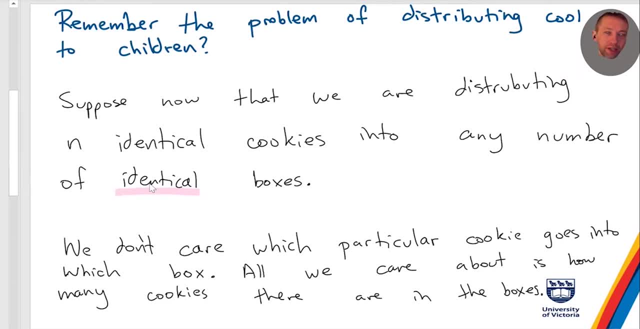 So remember this problem of giving cookies to children, right? So you have n cookies and you have k children And all the cookies are identical, right? And you wanted to break them up and give them to the children. You want to count how many ways there were to do that, right? And 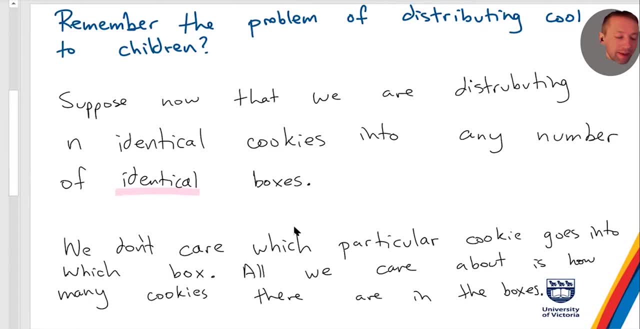 the answer was n minus one. choose k minus one if you wanted to give at least one cookie to each child. Now, giving three cookies to the first child and four cookies to the second child, or giving four to the first child and three to the second child, those are different things, right. 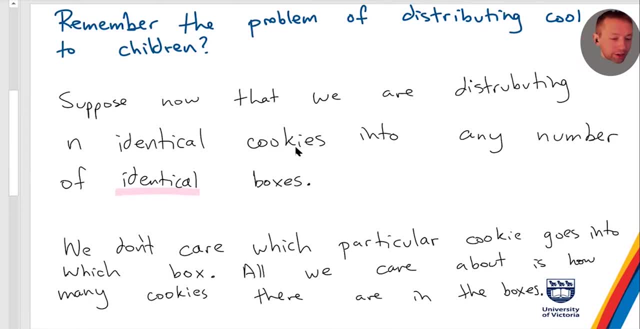 In that problem. But what if, instead of giving cookies to children- where children, you know every child is different- what if, instead, we want to put cookies into boxes where we can't tell the difference between two boxes? so the boxes are all identical. So imagine these are just. 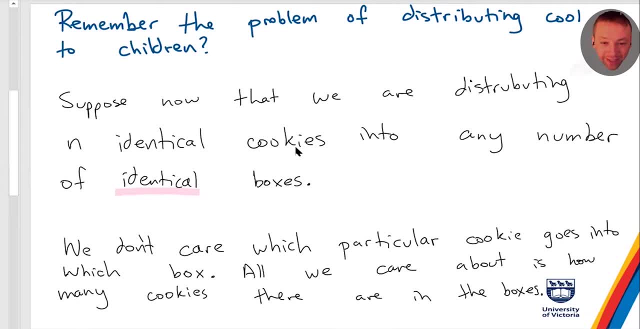 these like plastic boxes that you, you know they put cookies in at the grocery store or whatever. So I want to put you know, identical cookies into any number of identical boxes, And I don't care which cookie goes into which box, because all the boxes are the same. All I care is about is how. 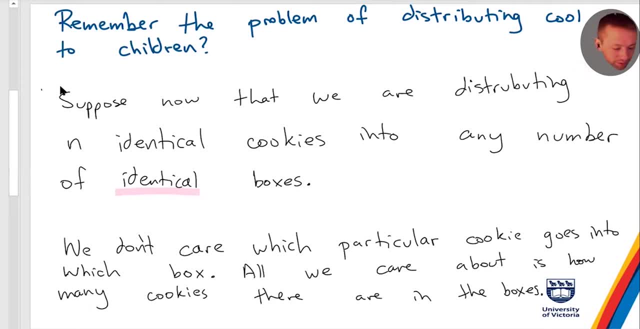 many cookies go into the boxes. So if I put two cookies in the first one and one in the second one, that's the same as putting one in the first one and two in the second one, because I can't tell the difference. So I want to put two cookies in the first one and one in the second one. 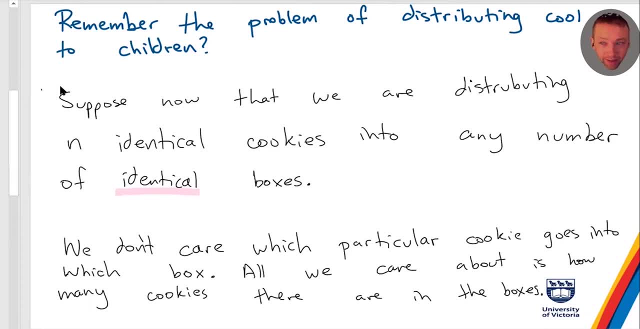 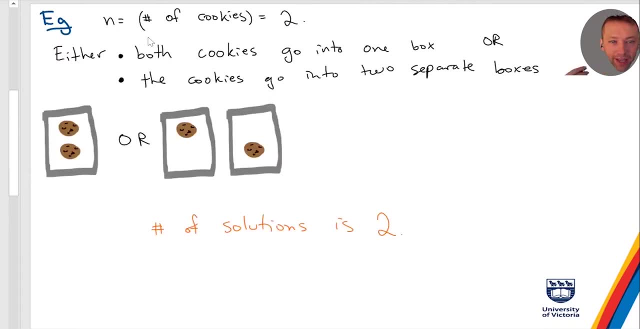 because I can't tell the difference, because I could just switch the boxes And it's all. you know, it's the same. So, to be clear, or I'm not sure if it is clear or not, But let's think about the case. 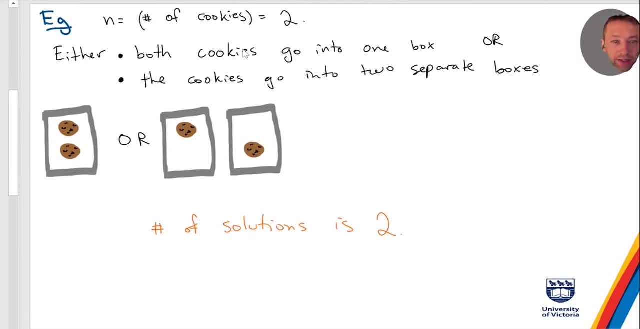 n is two, So n is the number of cookies. And let's say the number of cookies is two. So I claim that the number of ways to distribute the cookies is two, right? So either both cookies go into the same box, So that's one solution, Or you have the second solution, where the cookies go into two. 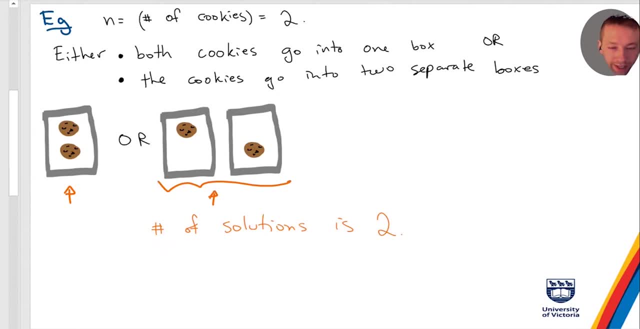 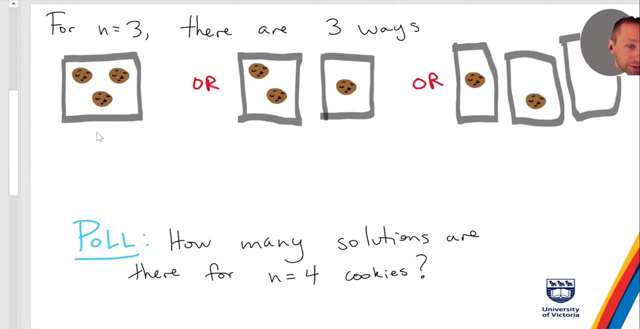 different boxes. Okay, I think it's a little bit more interesting when you go to three. So suppose you have three cookies, how many ways can I separate them into boxes where the boxes are all identical? And I claim that there's three ways to do it. So the first way is that I can put all of them into the same box. 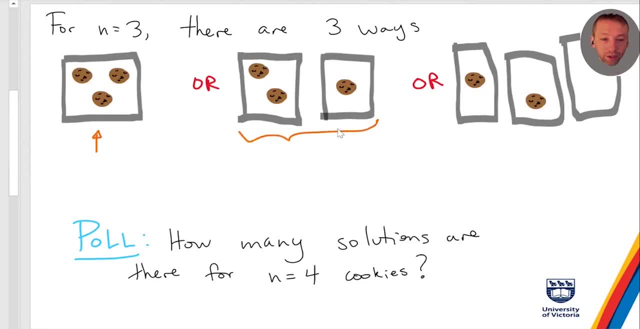 Okay, Or I could put: I could use two boxes, I could put two into one box and one into the other, Or I could use three boxes and I could put one in each. Okay, and notice that the answer here is 3.. 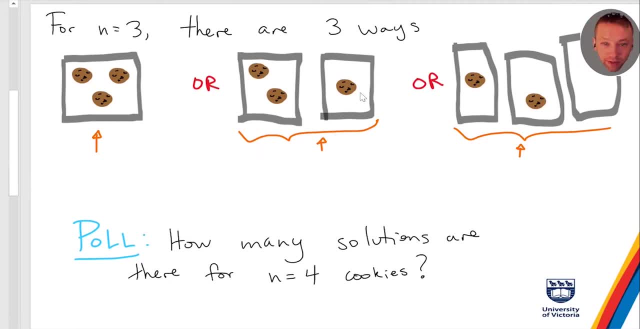 Not four. So if I put, you know, if I switch these two boxes, I consider that the same solution, because I can't tell the difference between the boxes. Is it clear what I'm saying here, that there's three solutions, not four? So if I put two in, you know one cookie in the first box. 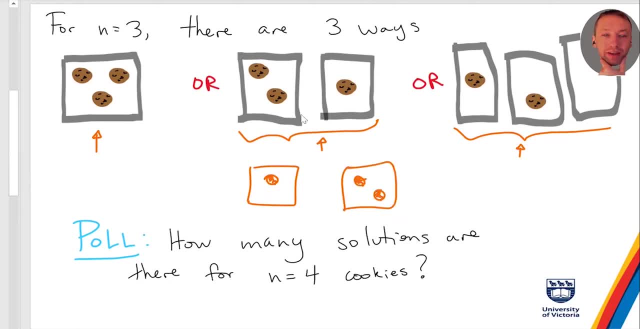 and two in the second one. I consider these to be the same thing because I could just switch the boxes and I wouldn't be able to tell the difference. So we want to distribute these identical cookies into identical boxes, so that, and we want to distribute them into identical boxes. 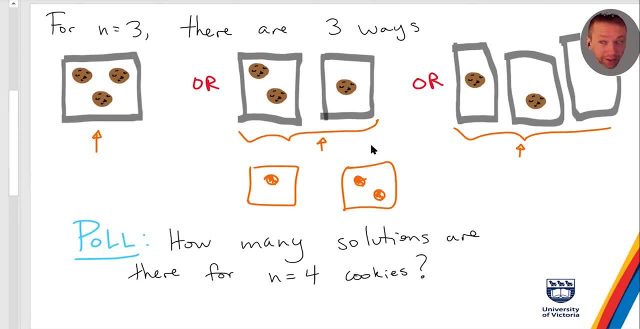 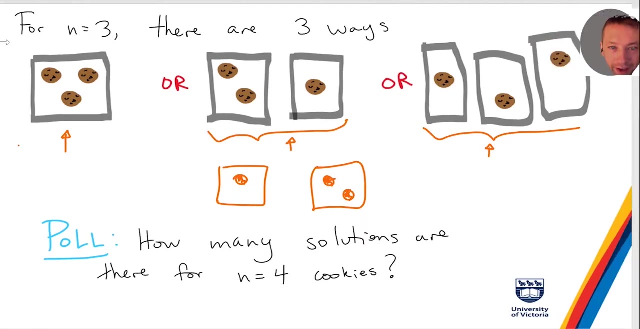 and we want to look at how many ways can I do that, And all I care about is how many cookies end up in the boxes. So so just to see if we understand this, let me give you a poll. So how many ways suppose I've got four cookies? how many ways can I do it? Okay, we're getting. 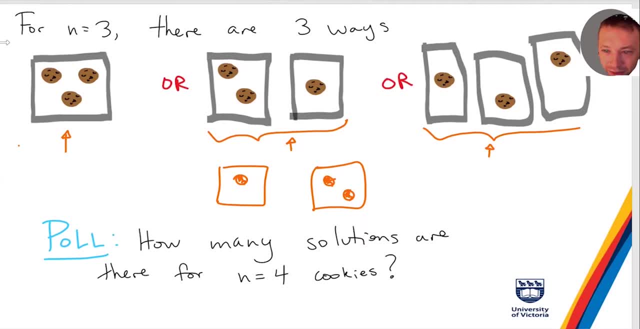 only a few answers so far. Feel free to give your opinion on this. The answers seem to be kind of clustering around a few different values. So is there four ways to do this? Okay, so I'm going to give you five ways to do it. five ways to do it. Some people maybe think there's six ways to do it. 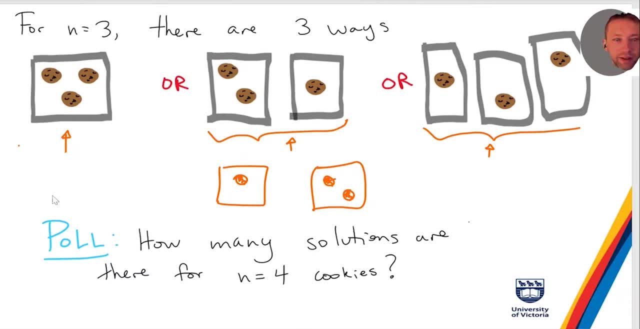 So okay, so well, let's kind of work it out. So if I want to put them all in one box, I have you know, I can. just there's only one way to put it in one box. I just put four in one box. 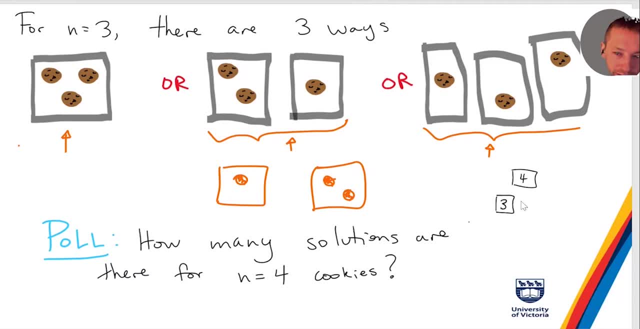 If I wanted to put it in two boxes, I could put three in one and one in the other. If I put one in the first box and three in the second box, that's the same thing, That doesn't count. as So I don't count one, three, because that's the same as three, one, I could put two in two. 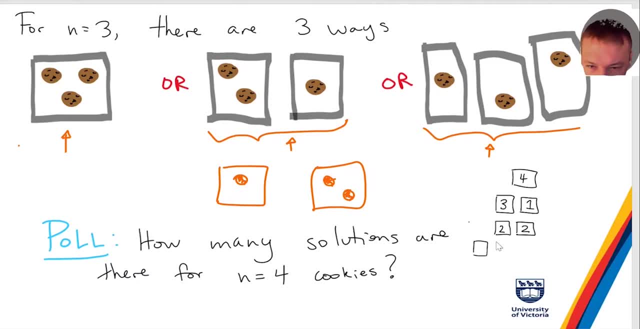 that's different. If I use three boxes, there's only really one way to do it. with three boxes, I could do two one one, Because if you think about it, if I any other way to use three boxes is going to be the same as two one one, And if I use four boxes I've got one one, one one. So 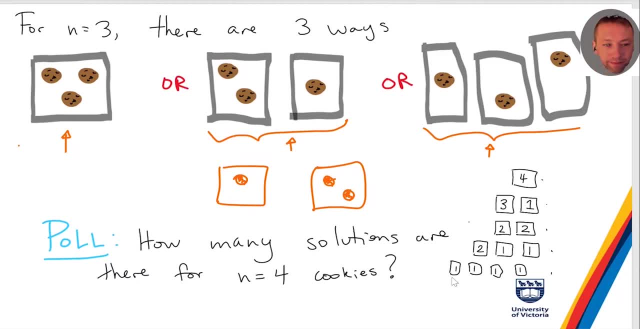 one, two, three, four, five ways to do it. So the answer is five. Okay, is that clear? Any questions about that? Did I miss one In particular? Okay, So, yeah. so this brings us to the next topic. 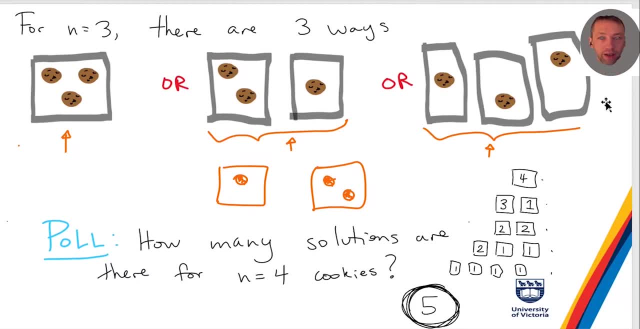 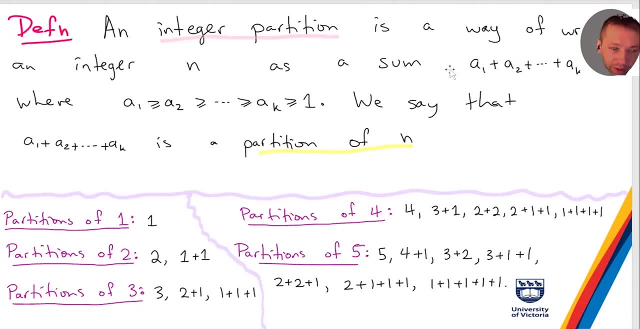 which is integer partitions. So an integer partition is a way of writing an integer n as a sum of numbers, a1 up to ak, where a1 is at least as big as a2, which is at least as big as a3,. 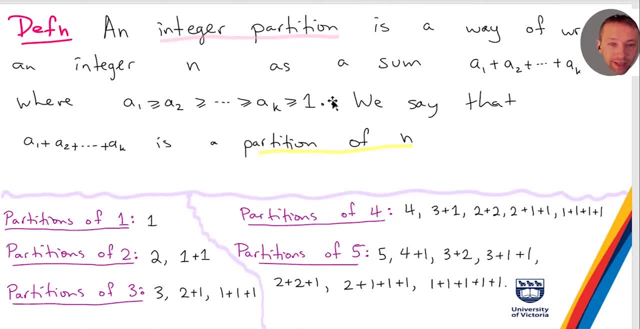 at least as big as a4,, etc. down to ak, which is at least one. So all the numbers are at least one And they come in decreasing order, And I say that. so the number, or I guess the notation I'll use for a partition is just: I just write the sum, So so I would say: 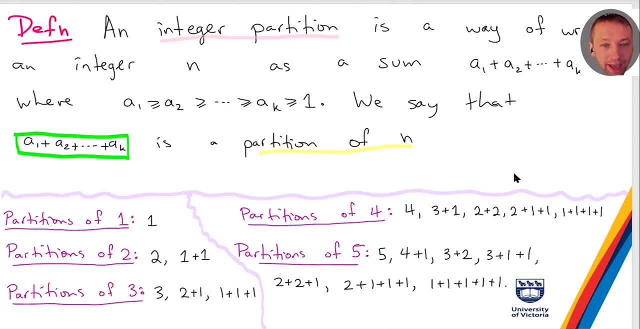 that a1 plus a2 plusetc, up to AK is a partition of n. So, for example, if I look at four, the number four, how many partitions are there? while I could take just four, the number four, right I? 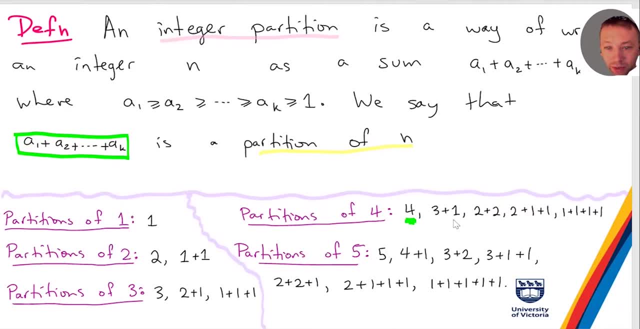 equals 4.. Or I could take: a1 is 3, a2 is 1.. So I take 3 plus 1.. Or I take 2 plus 2.. So those are all the partitions into two parts. So I call these things. by the way, these are called parts of the. 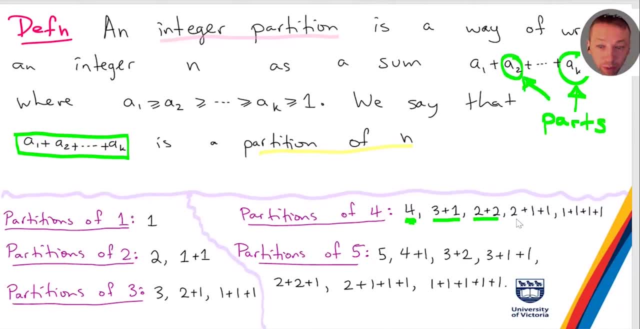 partition. So these are, you know, all parts. If I want to break 4 into three parts, I have 2 plus 1 plus 1.. And that's the only way to do it. Or I have 1 plus 1 plus 1 plus 1 into four parts, And 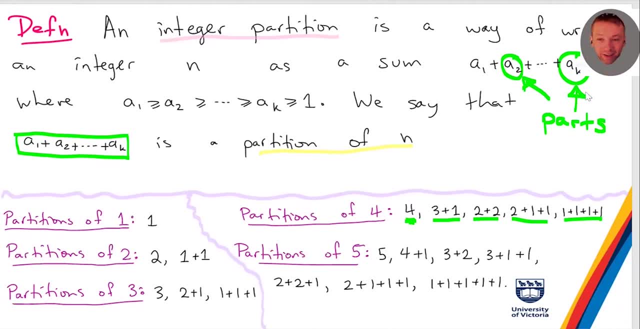 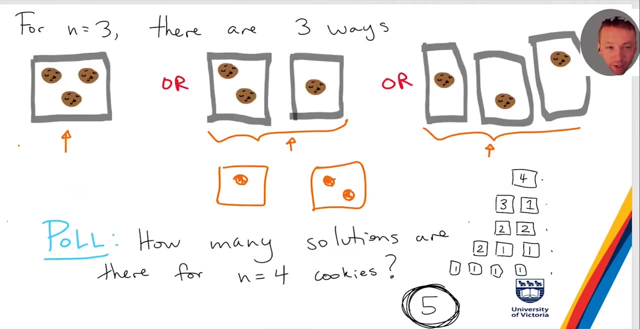 if you think about this, this is the same as this cookie question, right? Because all we cared about was how many cookies are in each box. We didn't care about switching the boxes, right? So actually, if you look back on the previous slide, these are basically writing out the partitions of 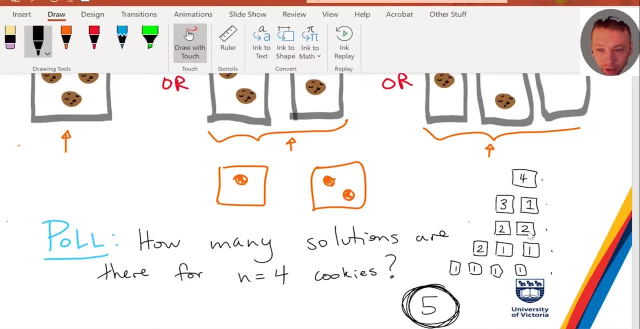 4.. So it's, I've got 4, I've got 3 plus 1,, 2 plus 2, or 2 plus 1 plus 1, or 1 plus 1 plus 1 plus 1.. 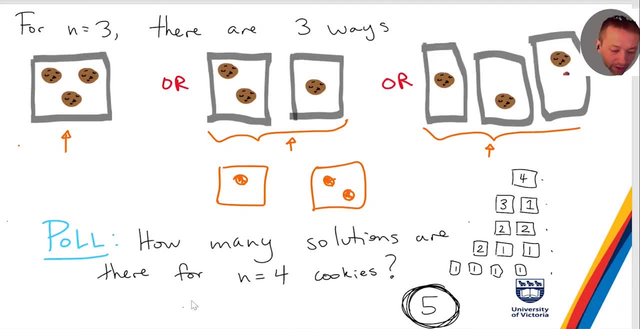 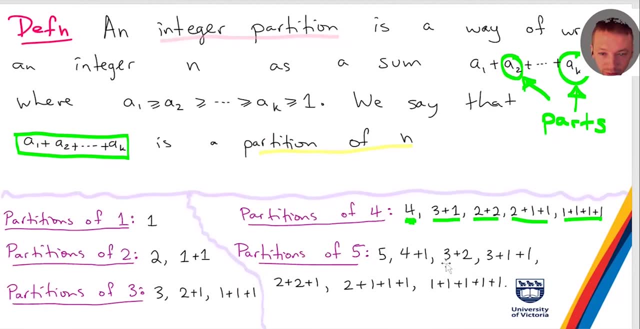 Okay, so the number of solutions to this cookie question is equal to the number of partitions of n. Okay so, partitions of 5.. So there's, I can do 5, or 4 plus 1, or 3 plus 2,. 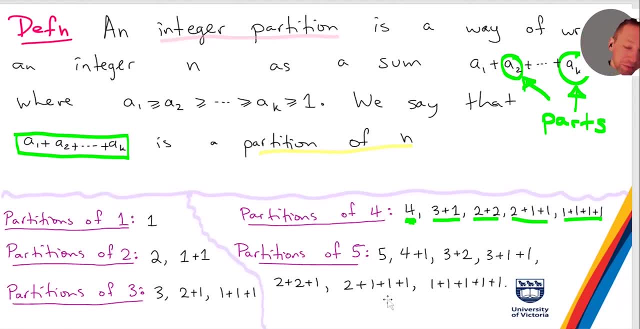 or 3 plus 1 plus 1,, 2 plus 2 plus 1, 2 plus 1 plus 1 plus 1, or 5 ones. So there's 1,, 2,, 3,, 4,. 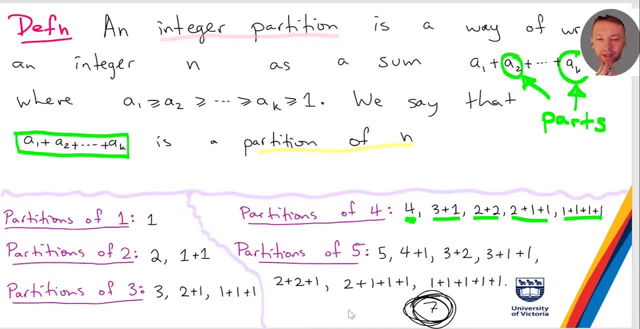 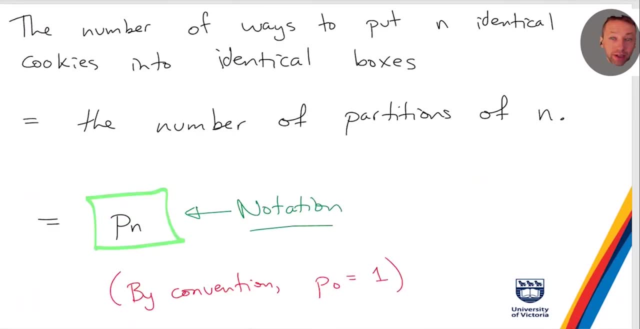 5,, 6,, 7 of them. So is it clear what a partition, an integer partition, is. Any questions about that? Yeah, so this is just kind of recapping what I said. So the number of ways to put n identical cookies into identical boxes. 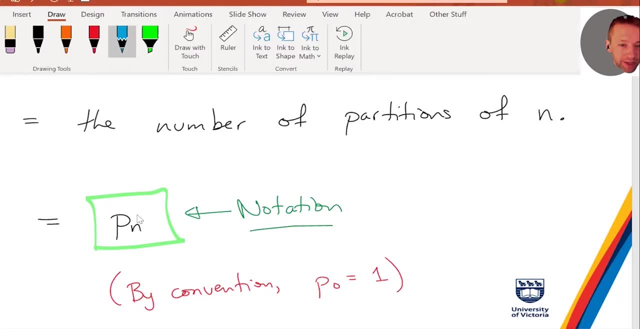 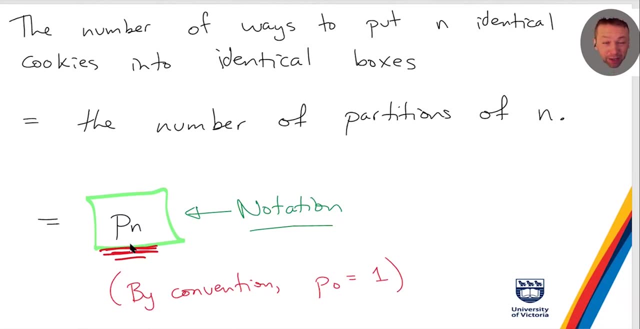 the number of partitions of n, and the notation we're going to use for this is pn. Now there's a bit of ambiguity if I talk about p0, like how many ways can I put 0 cookies into boxes, Just for convenience? it's always it's good to. it's going to be useful to think of p0 as being 1.. 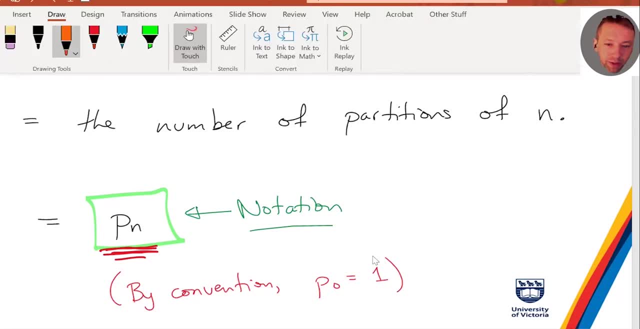 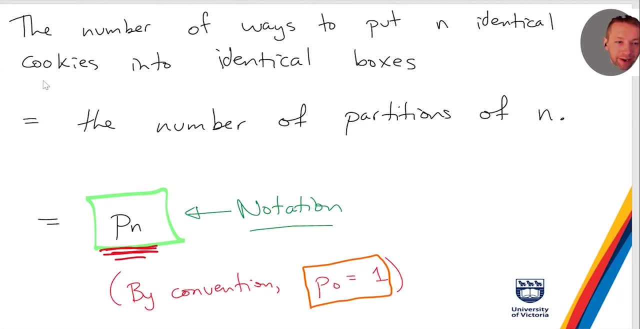 Okay, so don't worry too much about p0, but just remember that p0 is 1.. So the number of partitions of 0 is 1.. If you're, if I, anyone ever asks you, it's 1.. Okay, even though, yeah, maybe you could think there's 0 partitions. 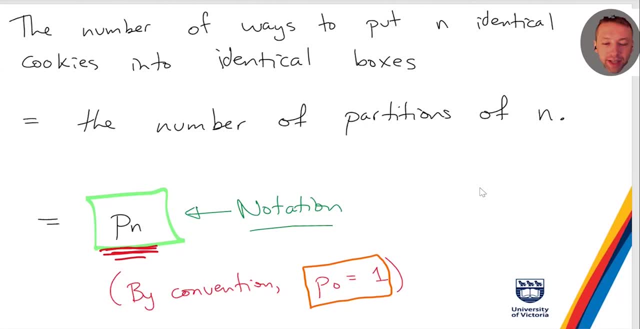 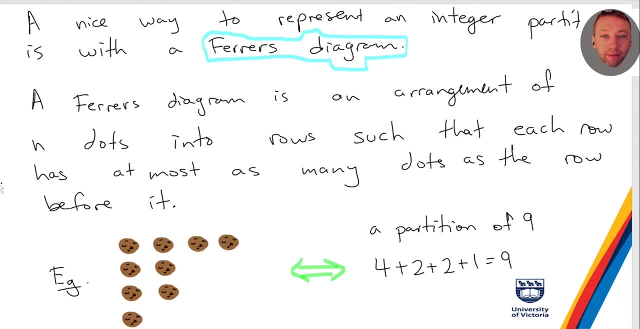 of 0, but let's just think of it being 1.. Okay, so pn is the partitions counts, the partitions of n. So there's a nice way of representing a partition which actually is going to immediately give us a theorem, by just kind of understanding this representation. So a Ferrer's diagram is an. 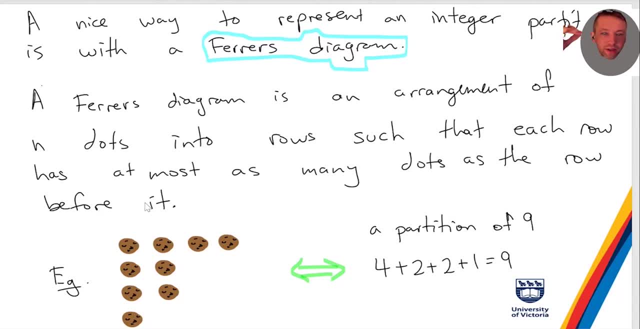 arrangement of n dots. So if I take the first row, I'm going to take the first row of n dots into rows so that every row, if I take the top row, okay, the top row has the most dots. The next row has at most as many dots as 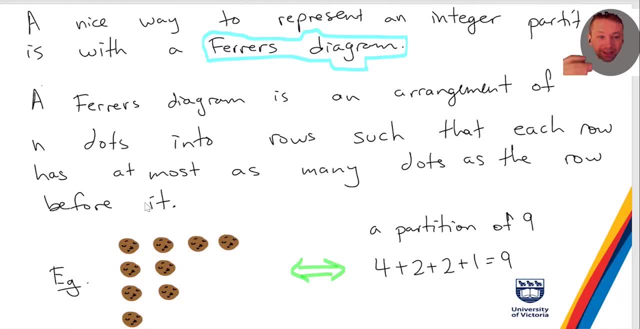 the top row, The third row has at most as many dots as the second row, and so on. So each row has at most as many dots as the row that came before it. So in total you have n dots. And yeah, you kind. 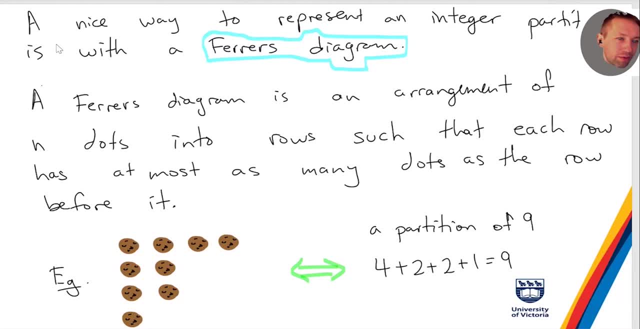 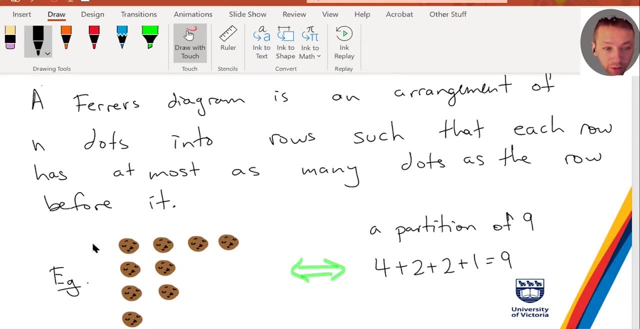 of arrange them in rows in this way. Now I think it's kind of clear that this is the same as a partition, Right? Because? so if I write down a Ferrer's diagram where I have 4 on the top, I have 2 on the next. 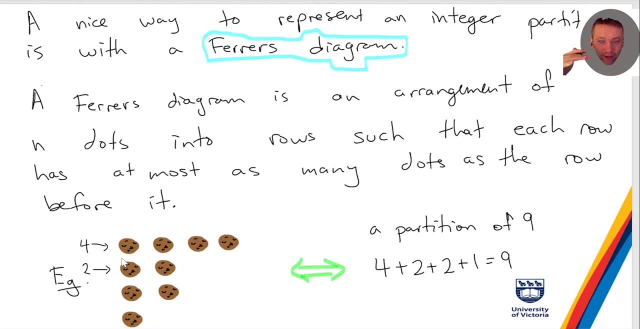 level, right. So a Ferrer's diagram you have to have. every row has to have at most as many as the previous row, but it could have the same number, right. So I could have 2 here and I have 1 here. Now it's kind of. 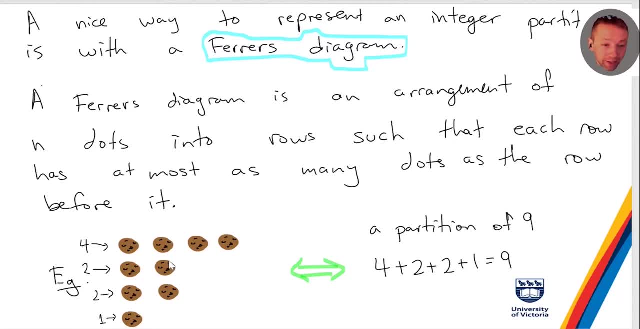 clear that this is the same as a partition of the number 9, because I've got 9 dots. If you add up 4 plus 2 plus 2 plus 1,, it's 9.. And this corresponds to the partition 4 plus 2 plus 2 plus 1.. Okay, But so note that we do this by rows, So the first row is the first number in the partition, not the first column. 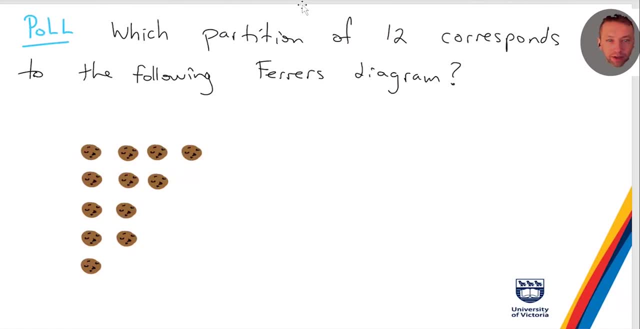 Let's do a poll, just briefly. So which partition corresponds to this Ferrer's diagram? So it's going to be a partition of 12, because in total you can see that there's 12 cookies. Okay, And, by the way, yeah in, usually if you see a Ferrer's diagram, they do that with dots, right? I don't know. I decided I'd already made this picture of a cookie, So I thought may as well do cookies. But yeah, if you look in the textbook, you won't see cookies. So think of these cookies as dots. But yeah, I think it's unanimous that everyone's got it. So it's going to be 4 plus 3 plus 2 plus 2 plus 1.. So the only way that you could. 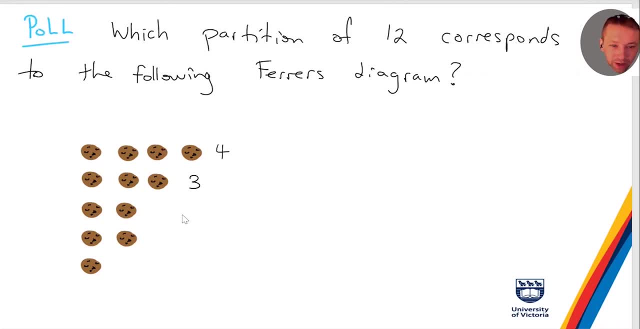 I think be confused on this is if you mixed up the rows and the columns, right? Because if I did it by columns, I would see: So yeah, so this is the answer: 4 plus 3 plus 2 plus 2 plus 1.. If I did it by columns, right, you could get messed up. So don't forget, it is by you know, you do the rows, not the columns. the columns would give you 5 plus 4 plus 2 plus 1, right, which is a different partition. But actually this observation about rows and columns is kind of a different partition. 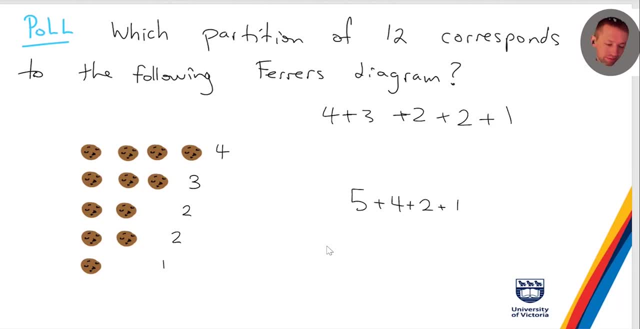 It kind of gives us something interesting Because I mean, the number of rows is the number of parts in the partition right, The number of columns is the biggest number in the partition. If you kind of take a transpose like if you know- I don't know if people know- kind of matrix transposes, but if you kind of take this picture and you flip it over the diagonal, you change the rows to columns and the columns to rows, then you get another partition of the number 12.. 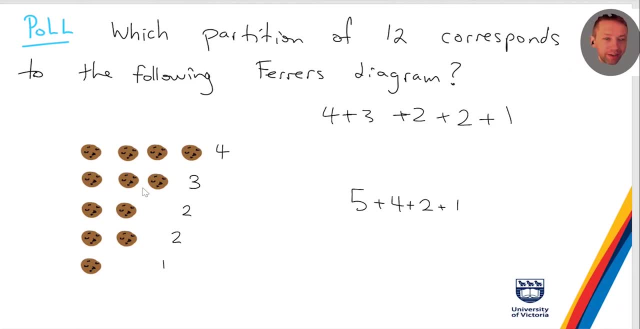 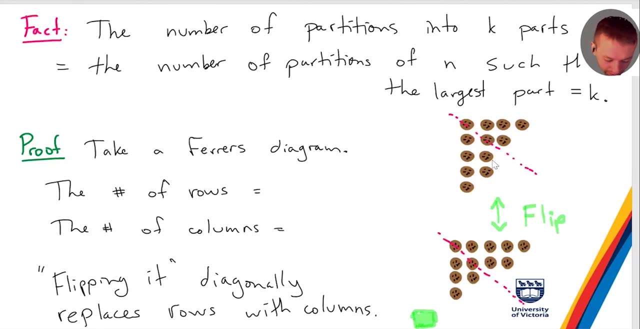 And this is the kind of a bijection between different types of partitions. So it's a- yeah, it's a kind of one to one correspondence, So let me kind of explain this more fully. So so the thing I want to tell you, using Ferrer's diagrams, is that the number of partitions into k parts is equal to the number of partitions. So this is a partition of n. So the number of partitions of n into k parts is equal to the number of partitions of n, such that the largest part is the largest part. 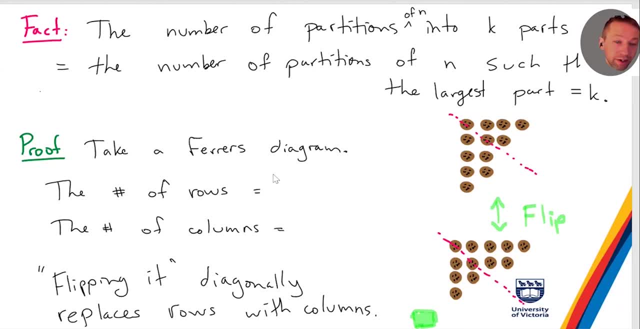 Is equal to k. And the proof is just to take a Ferrer's diagram. right, The number of rows in a Ferrer's diagram is equal to the number of parts in the partition. So if we're dealing with partitions into k parts, then it will be equal to k. The number of columns is equal to the. so if you look at, if you think of the number of columns here, it's just equal to what is the biggest element. So it's equal to the size of the largest part. If I take the Ferrer's diagram and I flip it diagonally, in other words, 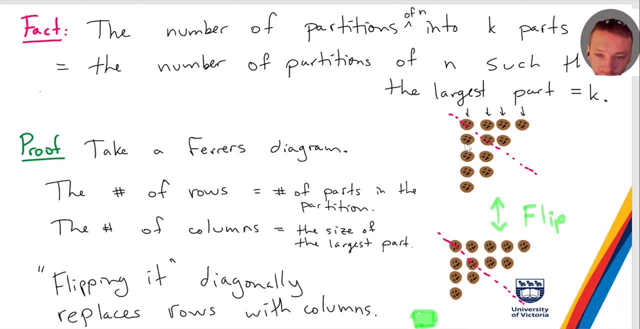 so flipping it diagonally is the same thing as saying: I look at the first column, which has one, two, three, four, five things, and I write it as a row. I take the second column and I write it as a row. I take the third column, I write it as a row, and the fourth column, I write it as a row. 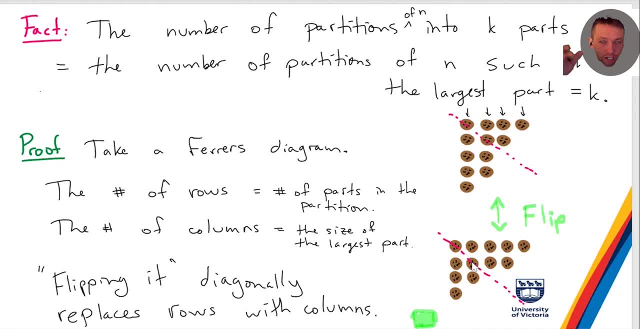 If you flip it this way, what's going to happen is the number of columns in your original partition or Ferrer's diagram will turn into the number of rows and the number of rows will turn into the number of columns. So this gives a number, a one-to-one correspondence. 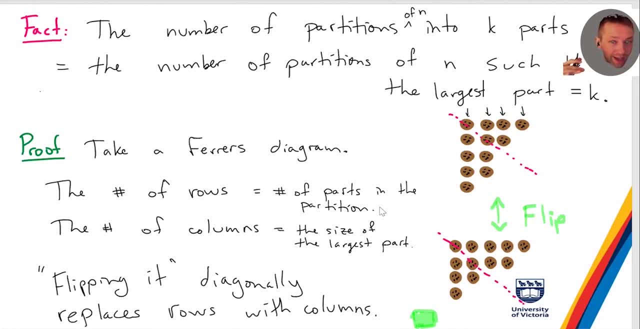 between Ferrer's diagrams where the number of rows is k and Ferrer's diagrams where the number of columns is k. In other words, it gives a one-to-one correspondence between partitions where the number of parts is k or the largest part is k. 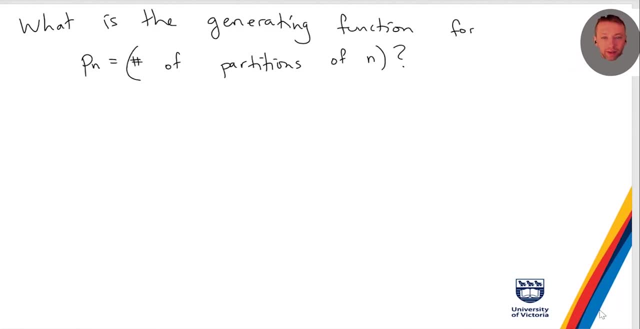 Any questions about this? Okay, so here's what we're going to do next, which is to come up with a generating function for partitions, which is a little bit tricky. So I want to find out: what is the generating function for Pn? 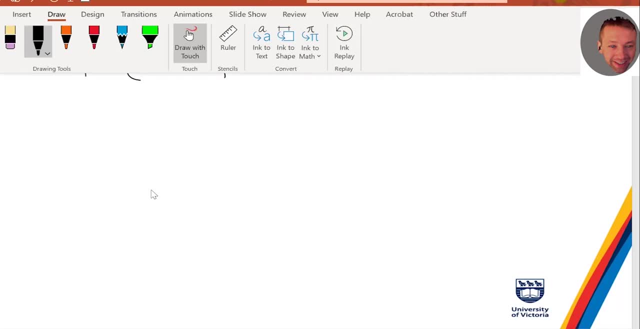 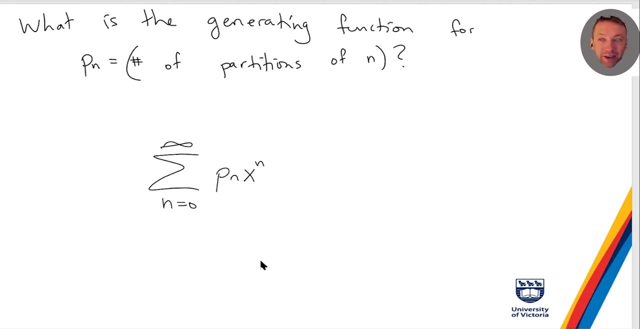 Okay. so on one hand it's pretty easy, because I don't know how to do it. I can just write that it's a sum n equals zero to infinity, Pn, x to the n. Okay, but that's not very useful. So I want to have a kind of more useful way of writing the generating function. 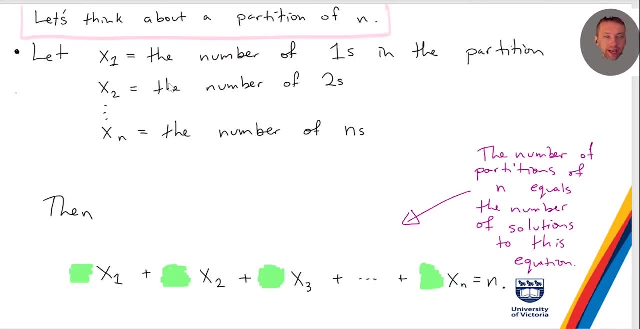 So let's think about a partition of n. So let's say I let x1 be the number of ones in the partition, x2 is the number of twos, x3 is the number of threes, and so on up to xn, which is the number of n's. 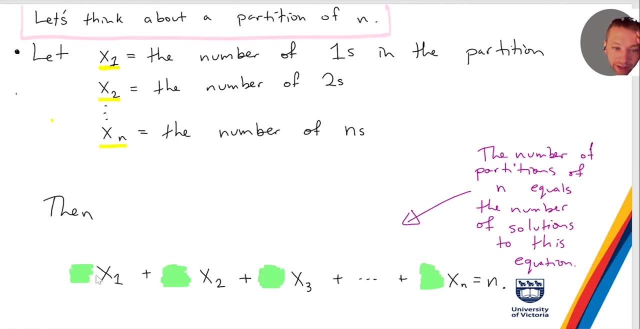 So what kind of equation can I get? What can I get involving these things? So I want to put a coefficient in each of these green blobs And I want to say that something times x1, plus something times x2,, something times x3,. 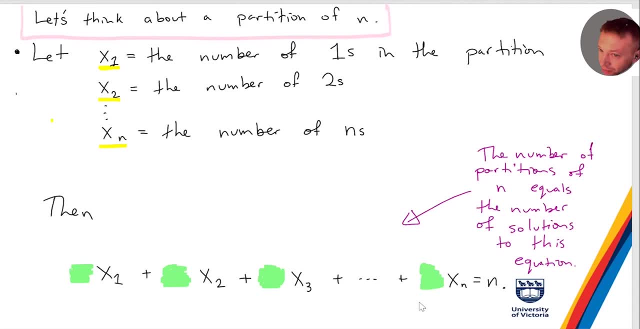 all the way up to something: times xn is equal to n for any partition of n. So if you think about it, the coefficient I want to put before each of these things is equal to the index. So if I take x1 times the number of- sorry, I take 1 times the number of 1,. 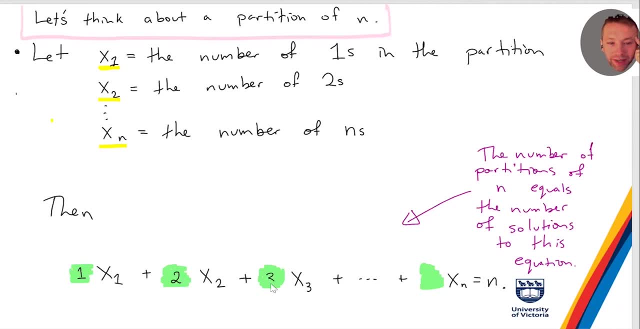 plus 2 times the number of twos, 3 times the number of threes, up to n times the number of n's in the partition, this equals n right, Because yeah, for example, if I'm taking 1 plus 1, plus 1, plus 2, plus 3, plus 7,. 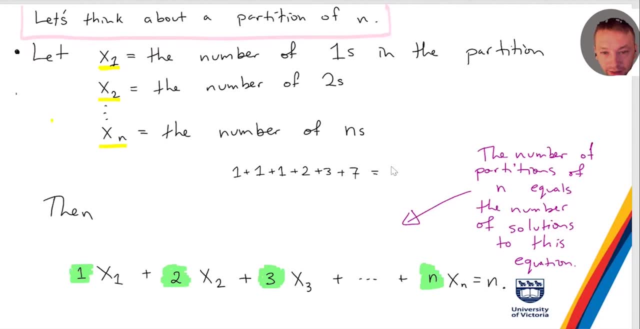 so that's 1,, 2,, 3,, 4,, 5,, 6,, 7,, 8,, 15.. So in this example I would have: x1 is 3, x2 is 1, x3 is. 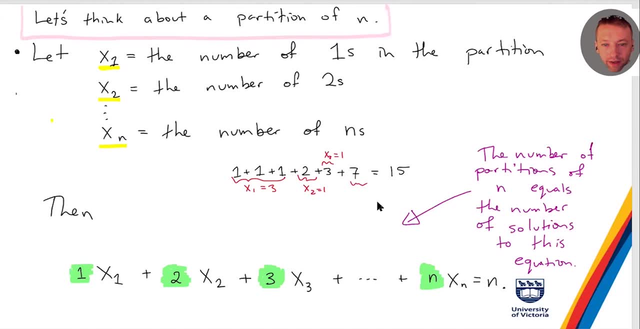 x1, x7 is 1, and all the other x's are 0. And if you check, you'll see that 1 times x1, plus 2 times x2, 3 times x3, plus 7 times x7, is equal to 15.. 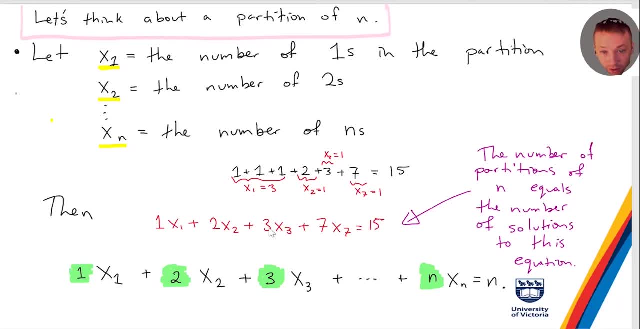 And here, implicitly, I have a 0 for all of the other terms because there are no other terms, right? So all of the other xi's are 0, and anyway, Right? so is this clear? So partition is equal to the number of solutions to this equation. number of partitions of n. 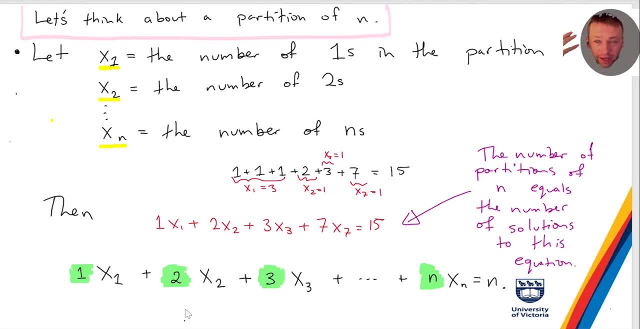 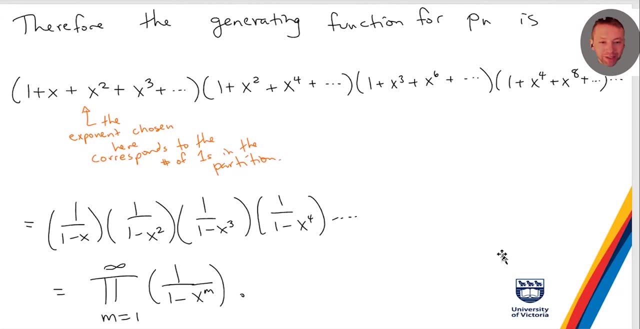 Okay so, using this, I want this to help me get a generating function for pn. Okay so, this is a little bit of a leap of logic here, but I need to, So I'll try to justify this. So I claim that the generating function for pn is like this: 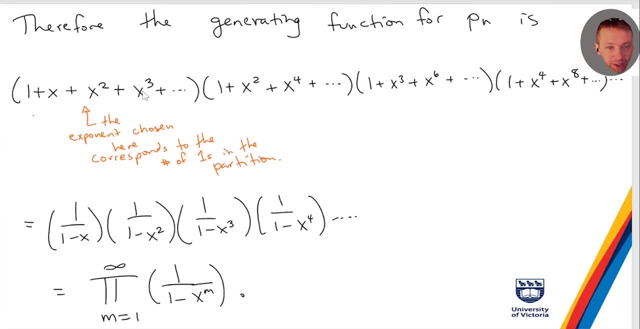 You take 1 plus x plus x squared, x, cubed, etc. off to infinity as my first factor. okay, And here the exponent that I choose will correspond to the number of 1s in the partition. So, using the notation from the previous slide, this is like: the exponent chosen here is corresponding to my x1,. 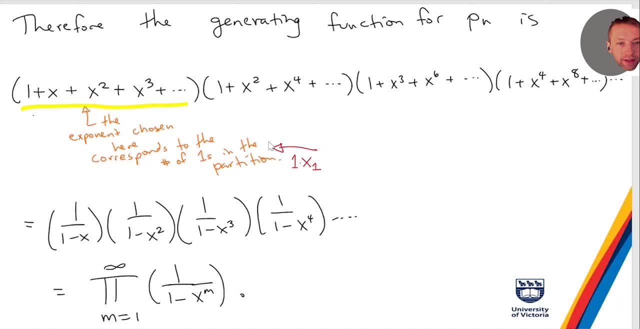 or 1 times x1, if that makes sense, Then I have 1 plus x squared 1 plus x to the 4, etc. And the exponent that I choose here to correspond to my x2 in some sense. So the exponent here is going to be my 2 times x2.. 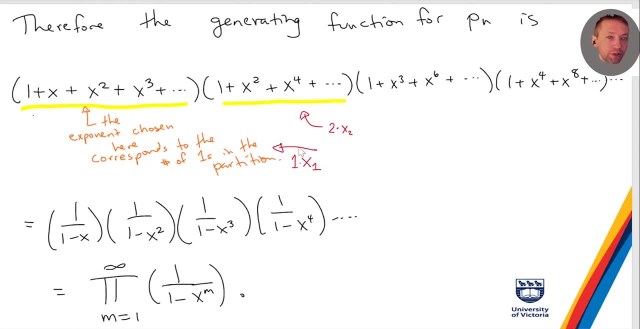 Or like it corresponds to the number of 2s I take in the partition, And the exponent here that I choose corresponds to my 3 times x3. And my exponent here corresponds to my 4 times x4, right? So I want 1 times x1 plus 2 times x2, plus dot, dot, dot, up to n times xn, to equal n right. 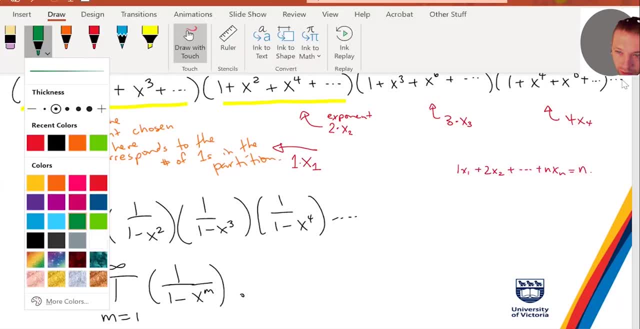 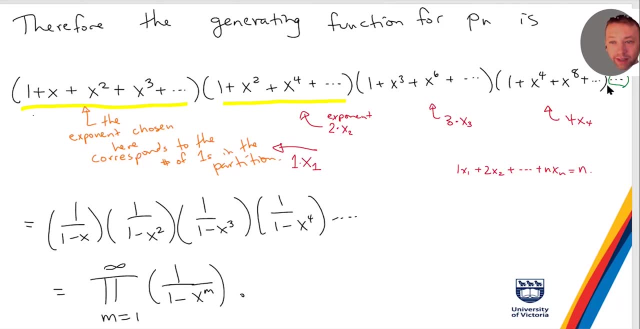 And here I've got a dot dot dot thing. because we do this, you know we keep this going, So we have 1.. The next factor is 1 plus x to the 5, plus x to the 10, and so on. 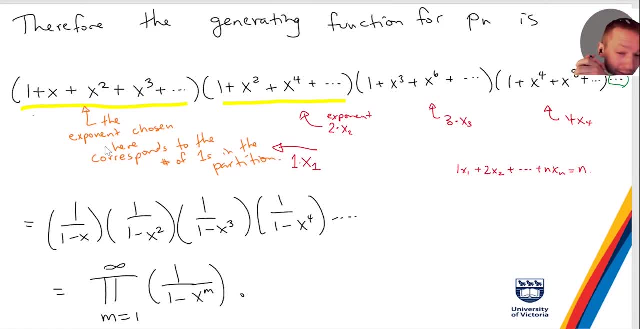 Okay, So if you think about it, it's a. I mean, it's a little bit maybe tricky to conceptualize this, But if you think about your coefficient- Coefficient of x to the n- The coefficient of x to the n will be equal to the solutions to this equation here. 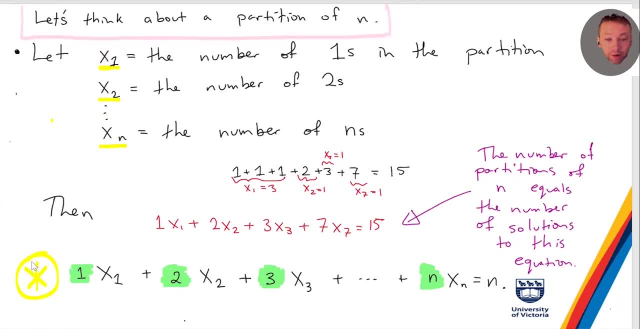 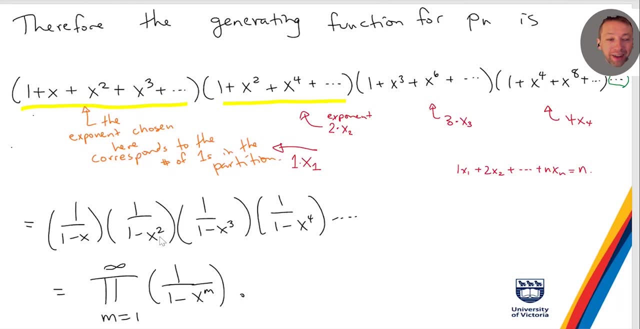 This equation, Which we've argued, is equal to the number of partitions of n. Now, of course, we know how to simplify this, Or I'm not sure if it makes it simpler or not, But the first term we can write is 1 over 1 minus x. 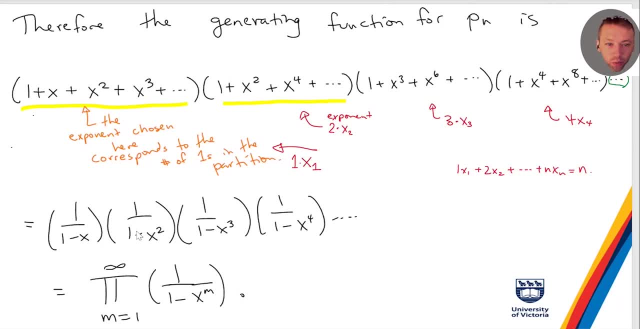 The second, Sorry, the first factor. The second factor is just 1 over 1 minus x squared. Then you have 1 over 1 minus x cubed, x to the 4. You know, x to the 5, and so on and so forth. 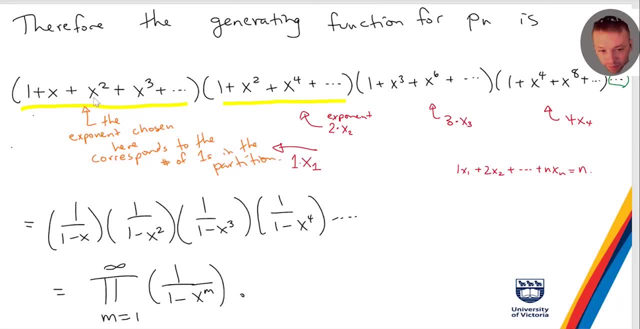 So this is just the product of. So I'm not sure, Are you guys familiar with this notation, This pi, This product notation? Yeah, So this is All I'm doing here is, you know, writing? This is just rewriting this. 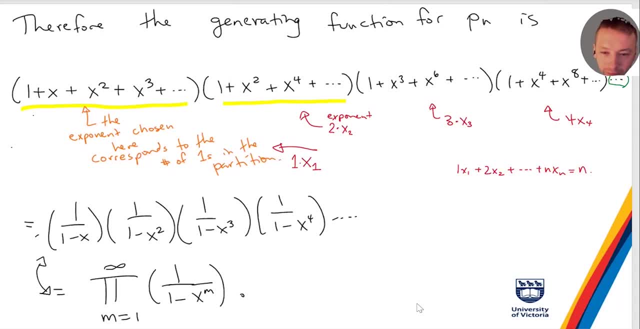 It's just the product. Okay, So let's say So this, This is: It's kind of like summation notation. Like you know, if I write sum of n equals 1 to infinity of an right, That's just the. 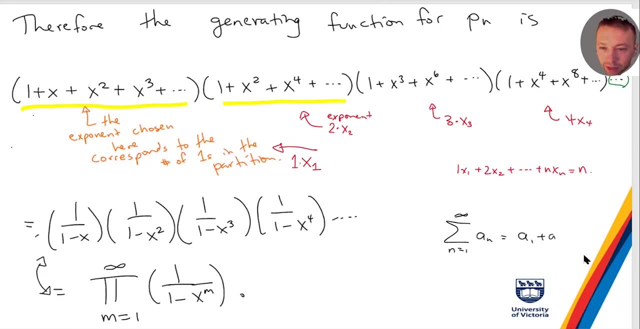 It's just the same as a1 plus a2 plus dot dot dot. If I write the product n equals 1 to infinity of an. it's like the same thing as the summation notation, except instead of summing you multiply. 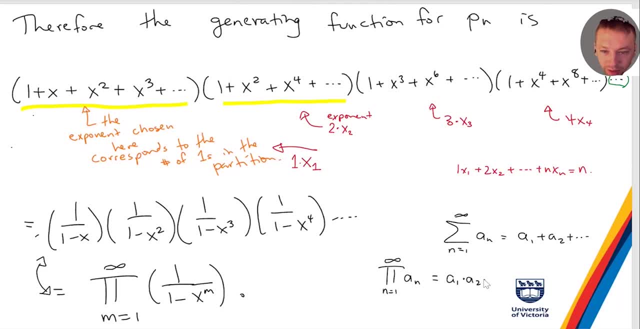 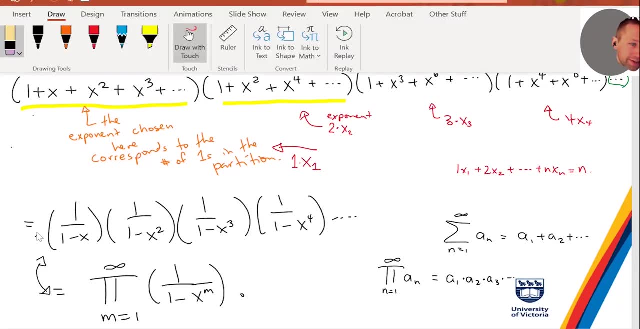 So that will be a1 times a2 times a3 times dot, dot dot all the way to infinity. So all I'm doing here is I'm rewriting, just because I don't It's a bit. you know, this dot dot dot is a little bit. 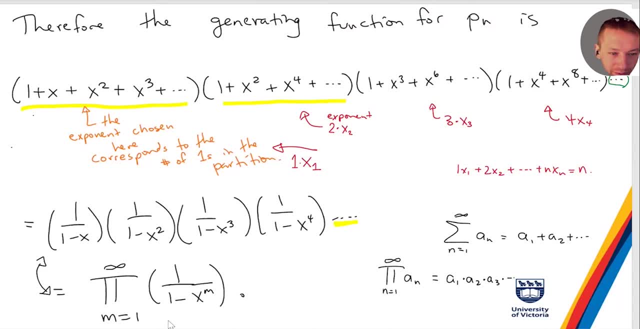 Not that formal, Just a little bit more formally. I'm just rewriting this like this: So the product m equals 1 to infinity of 1 over 1 minus x to the m. So which just means It just means the same thing as this. 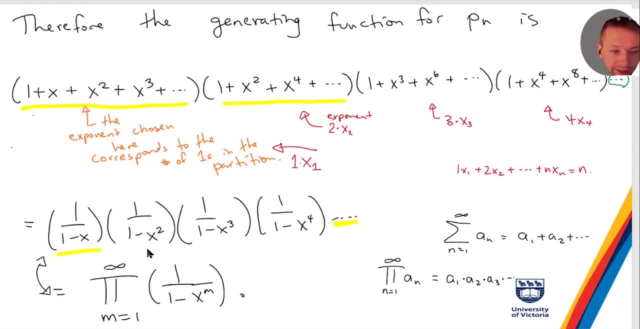 You take: m equals 1. So that gives you 1 over 1 minus x. m equals 2. That gives you 1 over 1 minus x squared. And then you just multiply them all up. So this weird thing is the generating function of partitions of n. 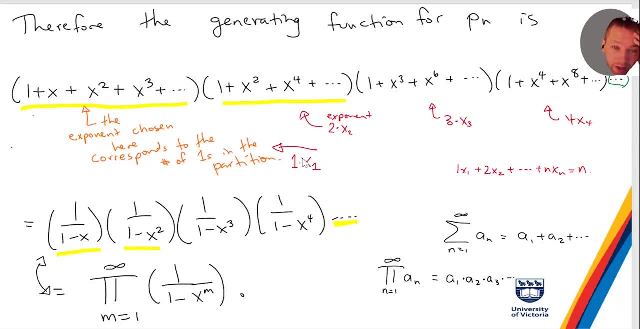 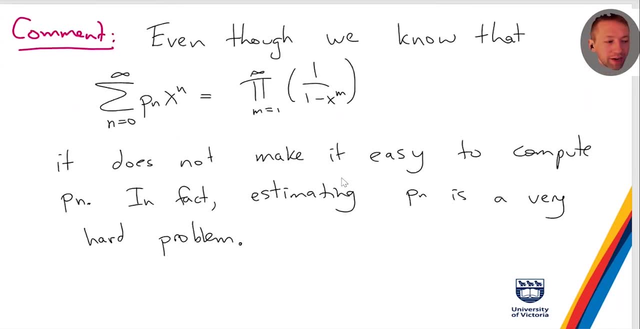 And yes, it is A kind of a weird function And I mean it's kind of also kind of a nice function. But even though it does give us a generating function for partitions in some sense, it doesn't actually make it easy to compute pn. 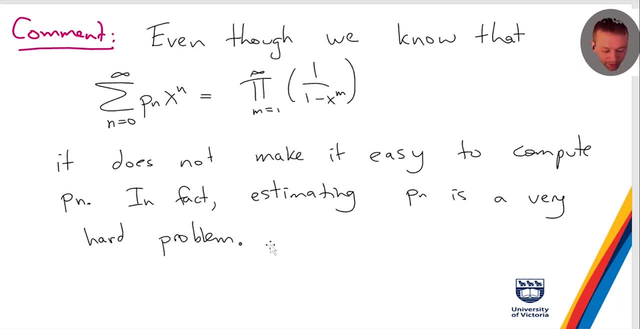 So this whole time we've been dealing with generating functions right And we've been. The great thing about generating functions has been that it allows us to compute numbers. In this case, this generating function isn't very good for computing pn, unfortunately. 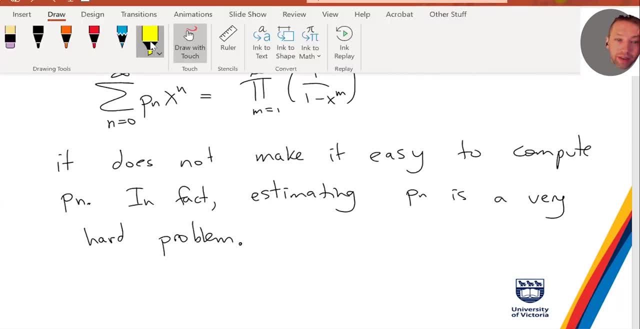 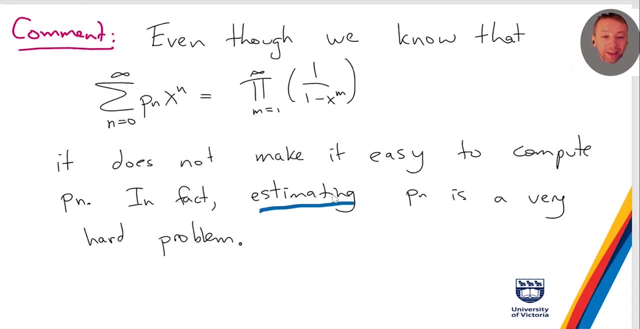 But nonetheless it is a generating function for it. But I should say that even kind of getting a rough idea of how fast pn grows, that's a very hard problem. So I think in the textbook it even mentions that in the movie The Man Who Knew Infinity.